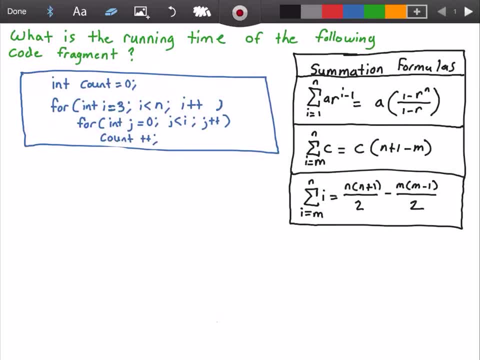 and then we have our outer for loop that states that integer i equals three, and it runs while i is less than n, so it never reaches n. Then we have i plus plus, which means that i increments by one each time. Next, within that outer for loop, we have our inner for loop, which states that j equals zero. 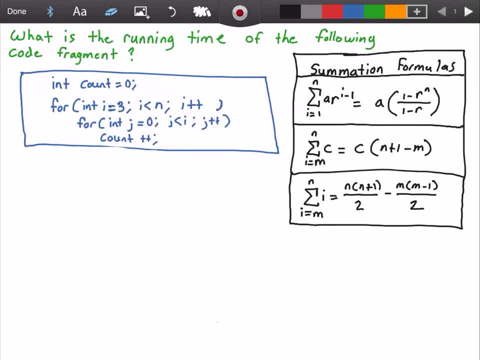 and it runs while j is less than i, so it never reaches i. and then we have j plus plus, which means that j increments by one each time. Now, within that inner loop we have count plus plus and that statement is going to be run some constant amount of time within our two for loops. 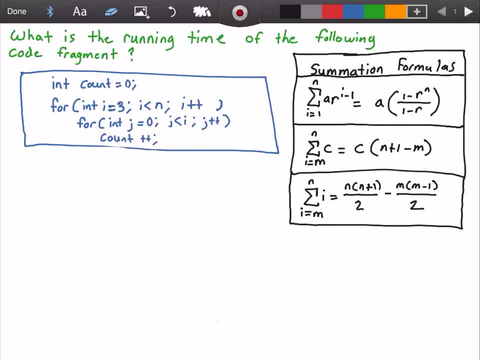 So let's get started And solve the running time of this code fragment using summations, since summations can represent for loops. So first thing I'm going to do is create a function called t, which will stand for time and it will take an input of size n, and I'm going to set this equal to the summation from: 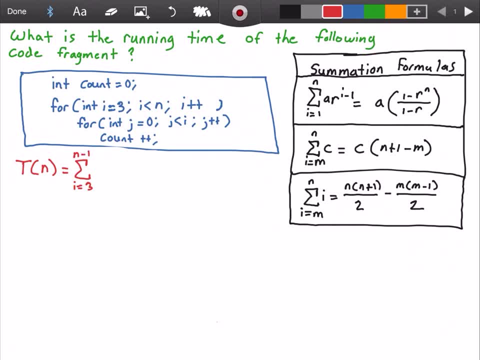 i equals three all the way up to n minus one, and this is because our outer for loop runs from i equals three to n minus one. i equals three all the way up to, but not including n right, because we have i less than n, so I have. 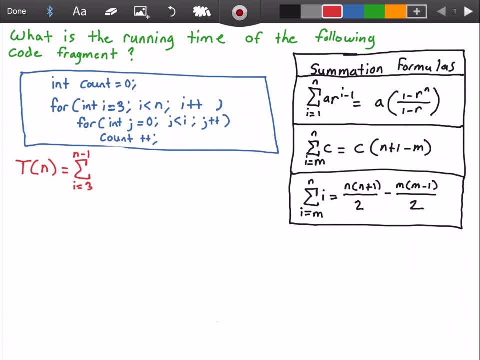 n minus one here. Next, within that outer for loop, we have another for loop that runs from j equals zero, and it's going to run while j is less than i. so within this summation, we're going to have another summation and this summation is going to run from j equals zero, like our inner loop. 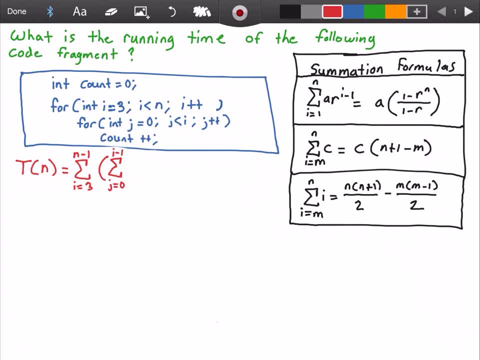 And it's going to run all the way up to i minus one, because it never reaches i. Now, within that second for loop, that inner for loop, we have our count plus plus statement, which is going to be ran some constant amount of time. so I'm going to use c for some constant. 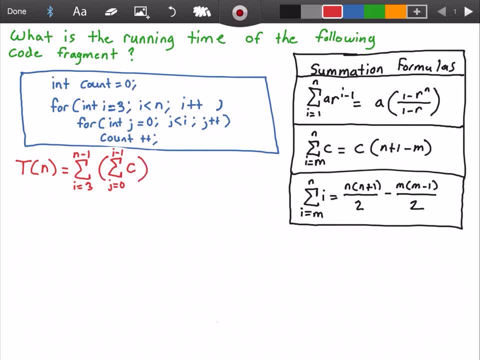 amount of time, and now we're done setting up our function. So what we can do is use some of these summation formulas to my right and the black rectangles to simplify this. So we're going to start by using this middle summation formula. okay. 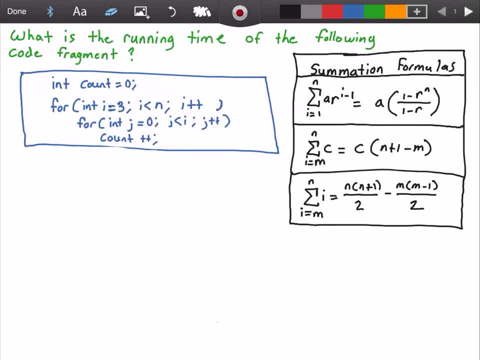 and it runs while j is less than i, so it never reaches i. and then we have j plus plus, which means that j increments by one each time. Now, within that inner loop we have count plus plus and that statement is going to be run some constant amount of time within our two for loops. 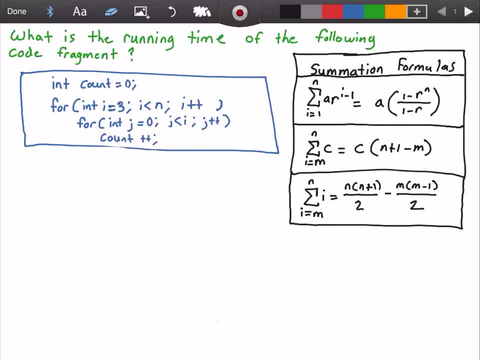 So let's get started And solve the running time of this code fragment using summations, since summations can represent for loops. So first thing I'm going to do is create a function called t, which will stand for time and it will take an input of size n, and I'm going to set this equal to the summation from: 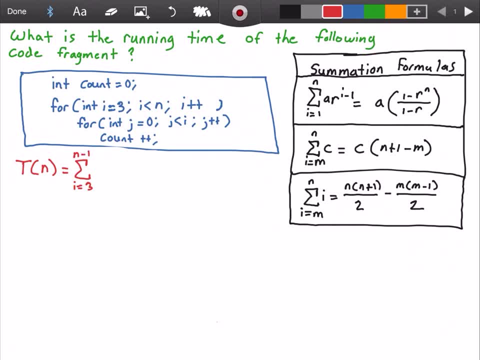 i equals three all the way up to n minus one, and this is because our outer for loop runs from i equals three to n minus one. i equals three all the way up to, but not including n right, because we have i less than n, so I have. 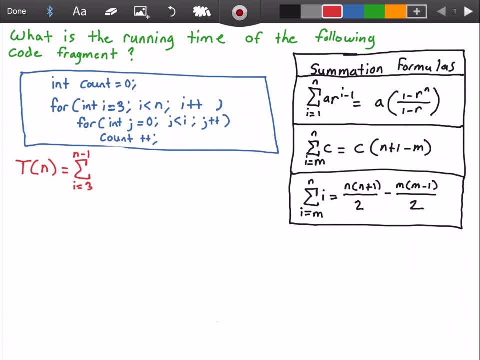 n minus one here. Next, within that outer for loop, we have another for loop that runs from j equals zero, and it's going to run while j is less than i. so within this summation, we're going to have another summation and this summation is going to run from j equals zero, like our inner loop. 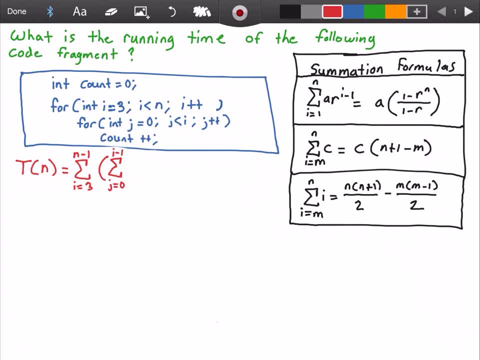 And it's going to run all the way up to i minus one, because it never reaches i. Now, within that second for loop, that inner for loop, we have our count plus plus statement, which is going to be ran some constant amount of time. so I'm going to use c for some constant. 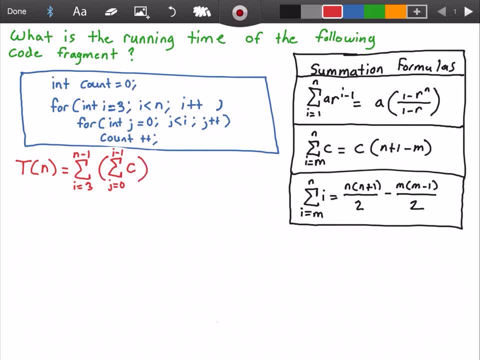 amount of time, and now we're done setting up our function. So what we can do is use some of these summation formulas to my right and the black rectangles to simplify this. So we're going to start by using this middle summation formula. okay. 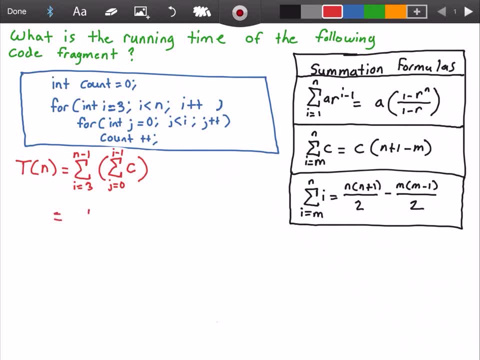 So let me go down here and I'm going to rewrite that outer summation. so we have the summation from: i equals three to n minus one, and using that second summation formula we get c times i minus one plus one minus zero. Okay, 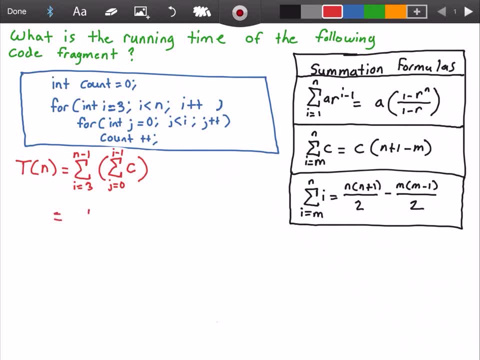 So let me go down here and I'm going to rewrite that outer summation. so we have the summation from: i equals three to n minus one, and using that second summation formula we get c times i minus one plus one minus zero. Okay, 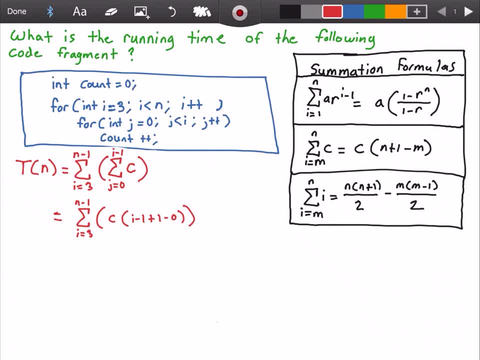 And if you're not sure how I got this, well, the variable n within the summation formula is equal to i minus one, and the variable m within the summation formula is equal to zero, and I just plug those values into our formula, okay? So let's simplify this. 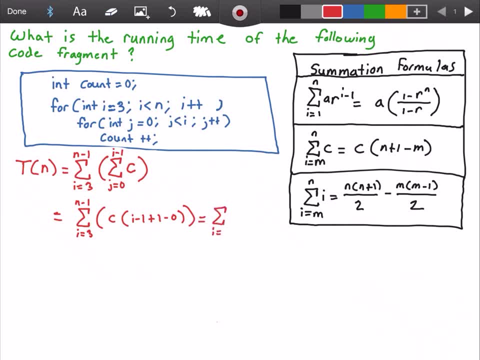 This is equal to the summation from. i equals three to n minus one. Okay, So let's simplify this. Okay, So we get n minus one of c times i. okay, and now, if we simplify this even more, we can just pull out that constant value or that constant variable, so we get c times the summation from. 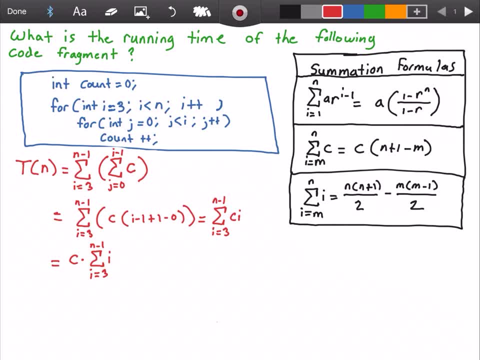 i equals three to n minus one of i, and now we can use this summation formula here at the bottom to solve for this. So this is equal to c times n minus one, times n minus one plus one, divided by two- and let me make sure I use my parentheses here- minus three times three minus one, all of that divided. 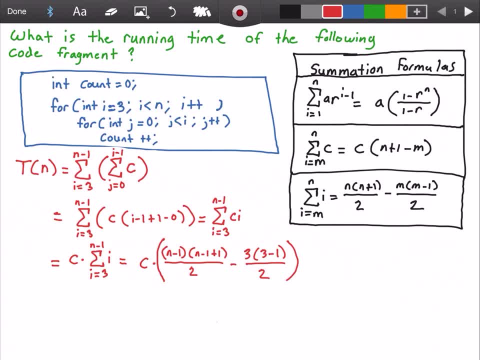 by two, Okay, And so let's simplify this a little bit. So this is equal to c times n minus one, times n over two- and again I'm going to use my parentheses- minus three, okay, So let's go down here, Okay. 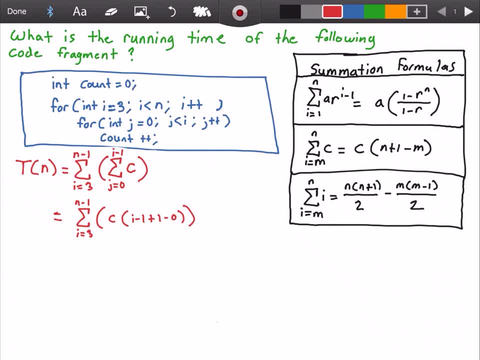 And if you're not sure how I got this, well, the variable n within the summation formula is equal to i minus one, and the variable m within the summation formula is equal to zero, and I just plug those values into our formula, okay? So let's simplify this. 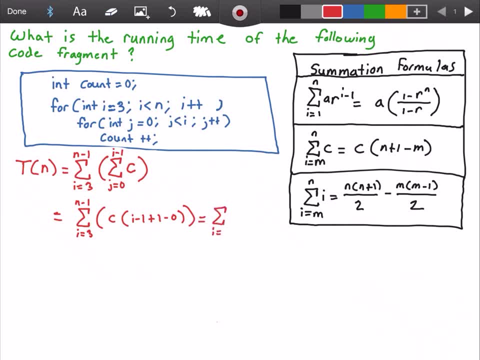 This is equal to the summation from. i equals three to n minus one. Okay, So let's simplify this. Okay, So we get n minus one of c times i. okay, and now, if we simplify this even more, we can just pull out that constant value or that constant variable, so we get c times the summation from. 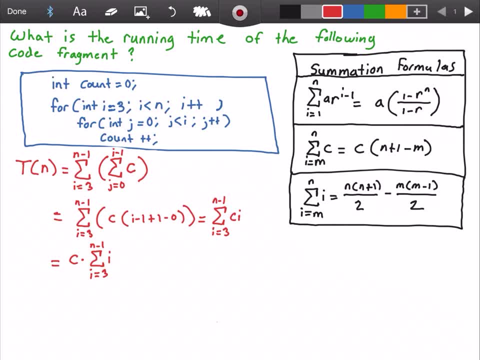 i equals three to n minus one of i, and now we can use this summation formula here at the bottom to solve for this. So this is equal to c times n minus one, times n minus one plus one, divided by two- and let me make sure I use my parentheses here- minus three times three minus one, all of that divided. 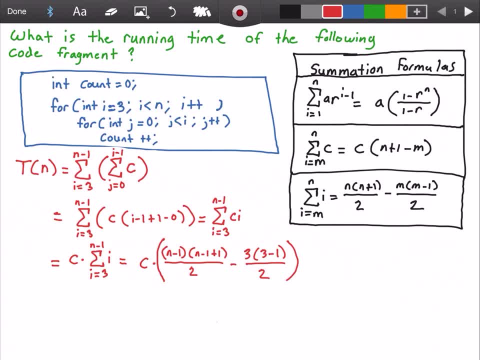 by two, Okay, And so let's simplify this a little bit. So this is equal to c times n minus one, times n over two- and again I'm going to use my parentheses- minus three, okay, So let's go down here, Okay. 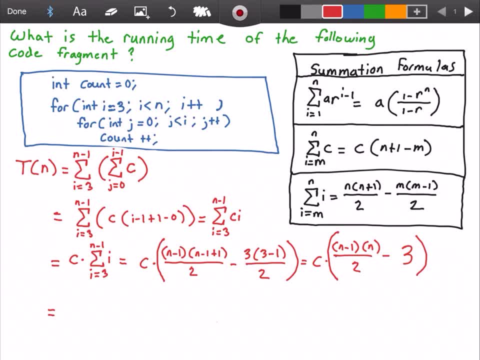 And we're going to continue to kind of simplify this a little bit more. So we get c times n squared minus n over two minus six divided by two, and this is equal to c times n squared minus n minus six, all divided by two. Okay, 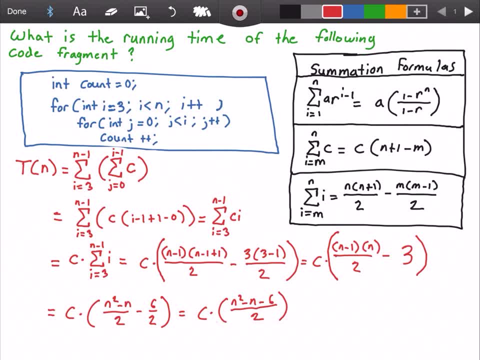 So this is our answer, and this implies that the code fragment is big O of n squared. Okay, Okay, Now, if you're not sure how I knew that and I knew this, you're going to have to look at another parameter that I knew. that I knew. 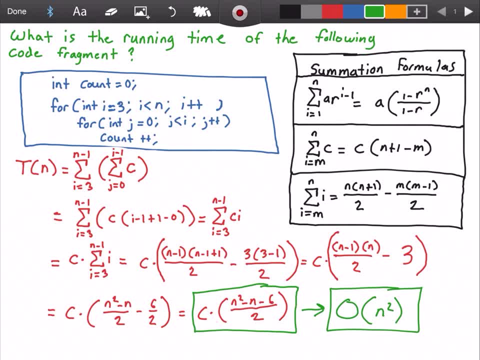 Okay, But number three, That number four, that this was big O of N squared. I just took the greater order of growth, which was N squared. but also I will put a link to a few of my videos explaining big O in the description below. so be sure to check those out and please leave any. 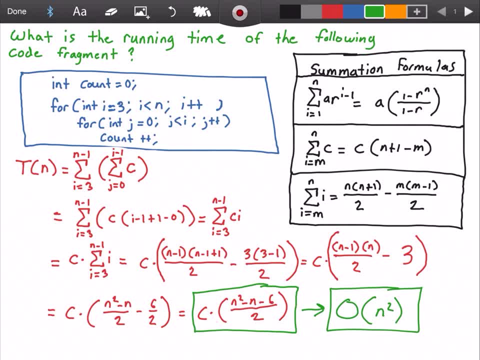 questions you have in the comment section. don't forget to hit that like button and that subscribe button and if you found this video helpful, please share it. maybe others will find it helpful as well. and that's basically it. thank you for watching and I'll see you all in the next video. 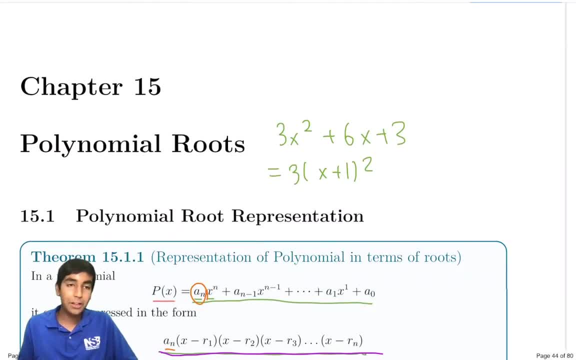 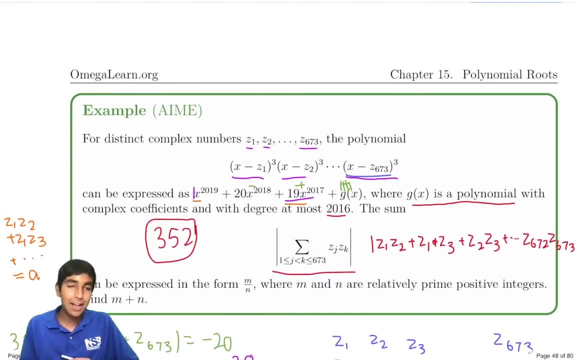 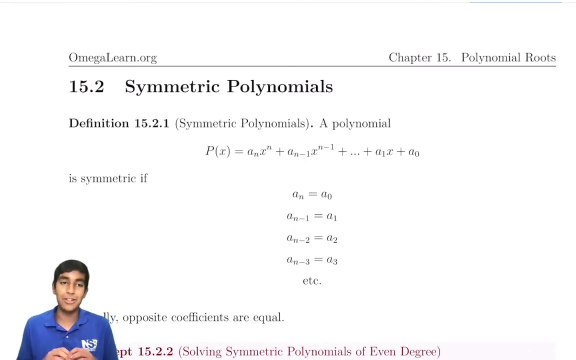 Last time, on Mastering AMC 1012,, we covered the polynomial root representation and how it can be used to simplify even the hardest of problems, from USAMO and AAMI to something that's easily solvable. Today, we're talking about symmetric polynomials and polynomial manipulations. 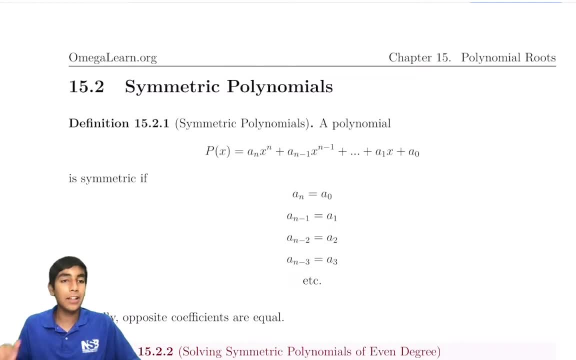 and we'll see how this could make a problem that's hard to solve with Viettas easy by just changing the polynomial. So, first of all, what is a symmetric polynomial? A polynomial with coefficients equal on both sides. Here's an example of one: 3x squared plus 6x plus 3, because 3 is equal to 3 and 6. 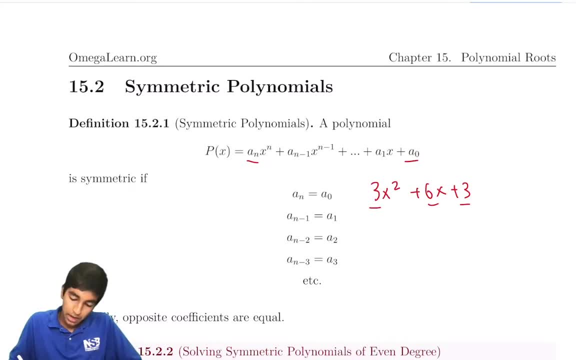 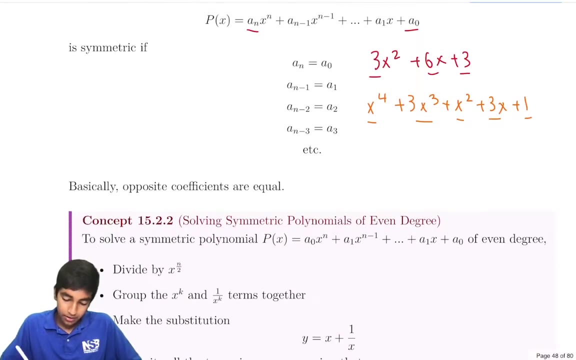 is well equal to itself. It could also be bigger, like this: 3x cubed plus x squared plus 3x plus 1.. 1 is equal to 1,, 3,, 3, and 1.. Okay, so now that we know what.